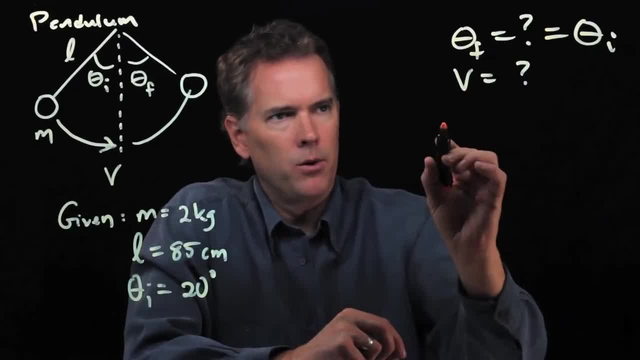 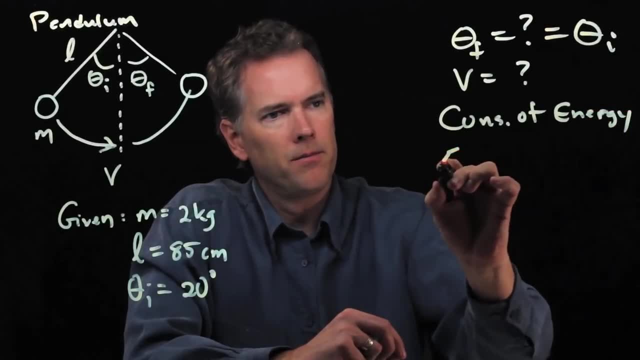 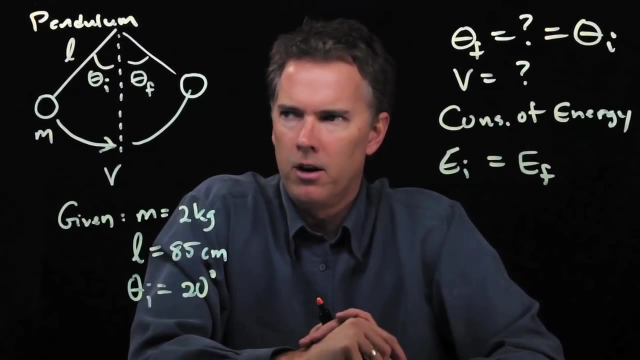 All right To get v. we're going to use conservation of energy and the initial position is going to be where it starts. The final position is going to be at the bottom. okay, So E i equals E, f, E i is all gravitational potential energy, okay. 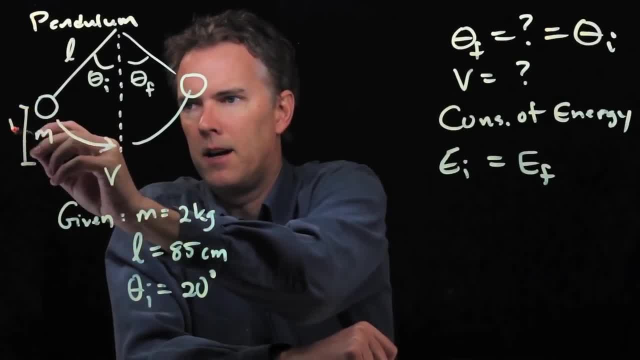 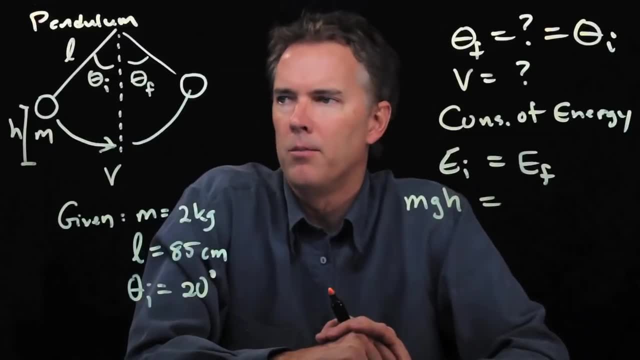 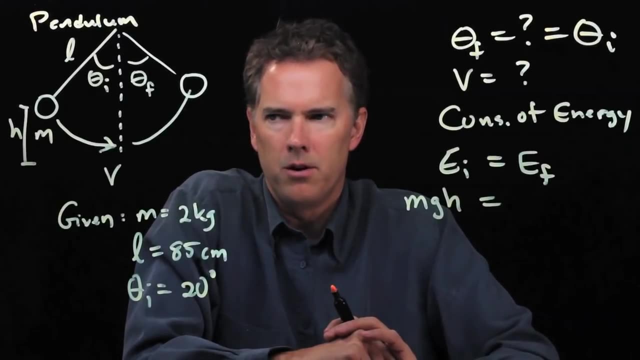 It is up here at some height h and we need to write down what the gravitational potential energy as a height h. It's, of course, just mgh Down. at the bottom it's at a height zero. That's where we're going to set our height equal to zero. 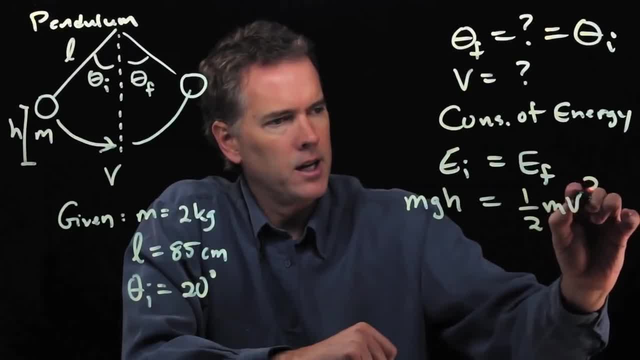 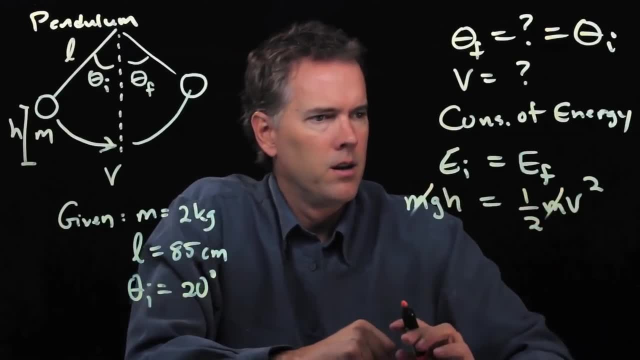 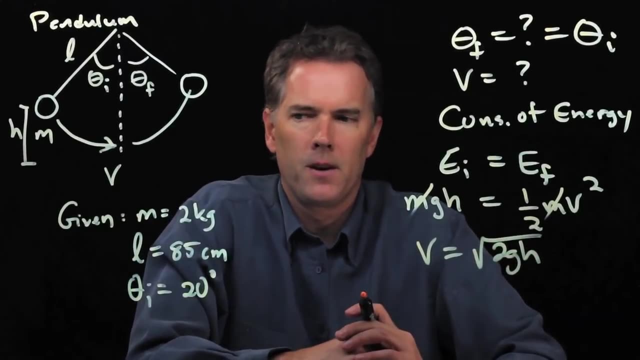 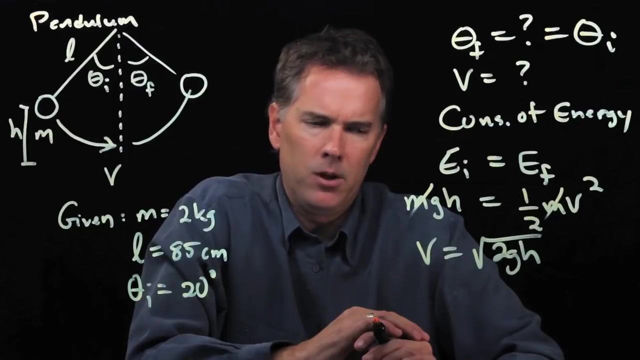 And we know it is moving, so it has kinetic energy one-half mv squared. All right, We could solve this for v, The m's cancel out. We get v equals square root 2gh. okay, It's nice, We didn't even really need the mass in this calculation, But we don't really have h right. 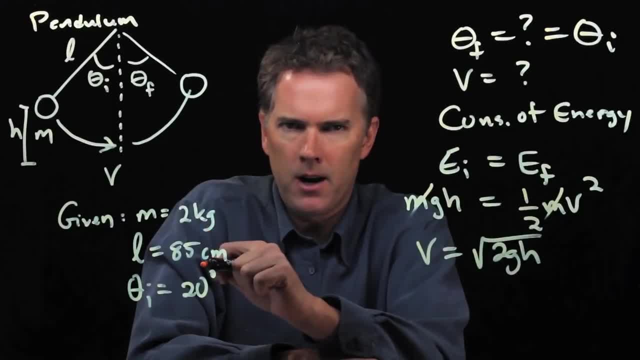 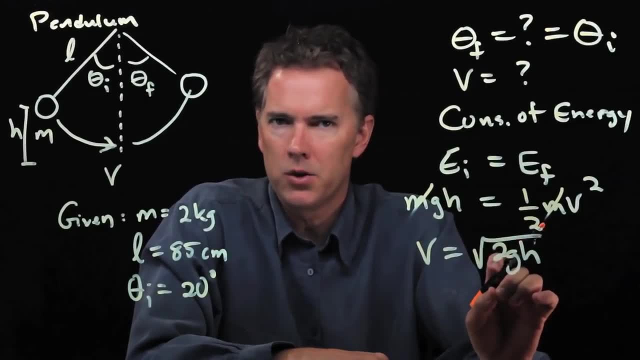 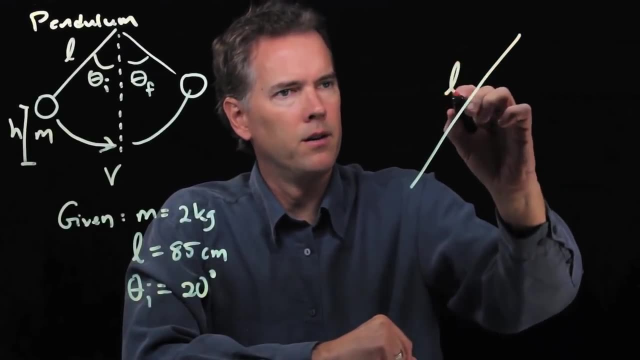 We know l and we know theta And we know theta i, so we need to combine those somehow to get h. So this is slightly tricky, but we can do it. Let's redraw this triangle just a little bit bigger. This is l. 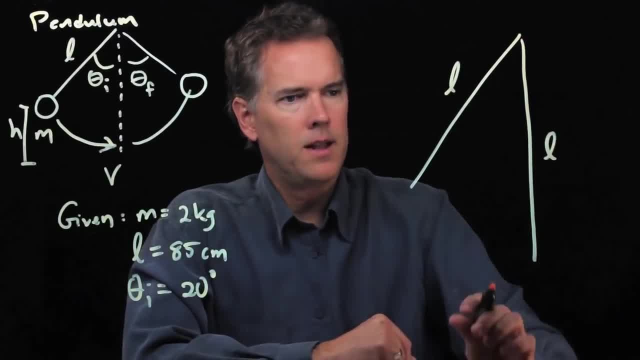 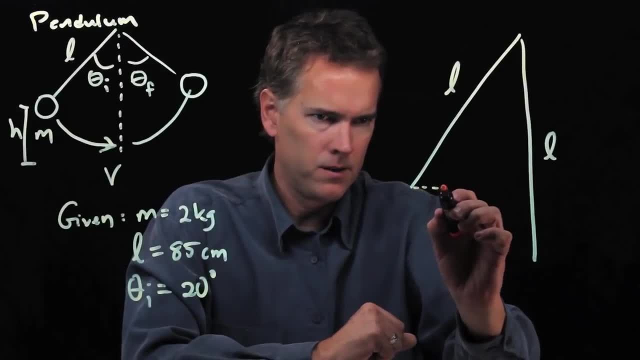 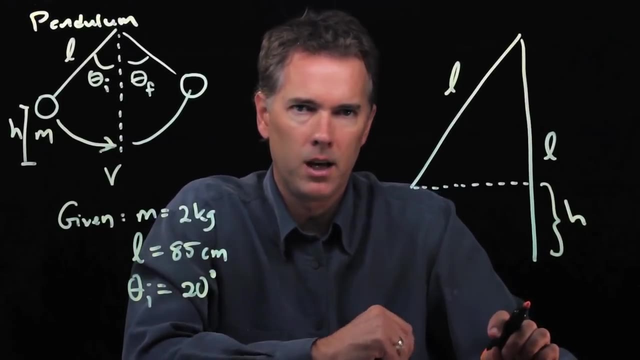 When it's at the bottom, that's also l. okay, It's the same string, And so the height that we want is this, right here, That little section h. okay, That's how high it is above the ground when it starts. 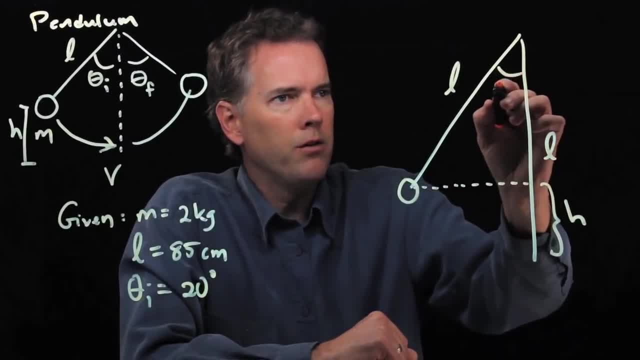 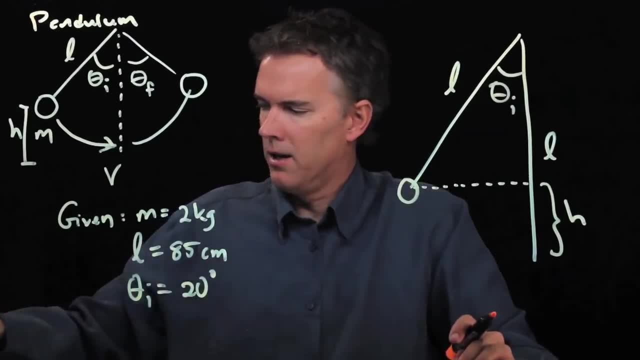 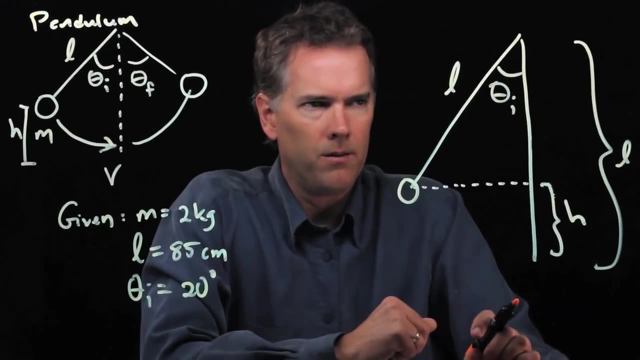 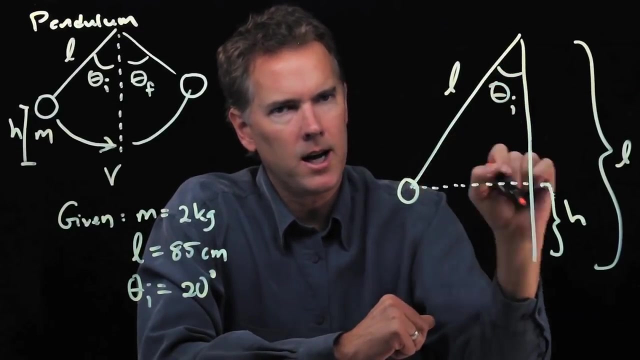 There's its starting point. What do we know? We know this theta initial, okay, And we know that the whole length of the string is l. That whole length is l. So if we knew this section right here, then we could calculate what the height is. h. 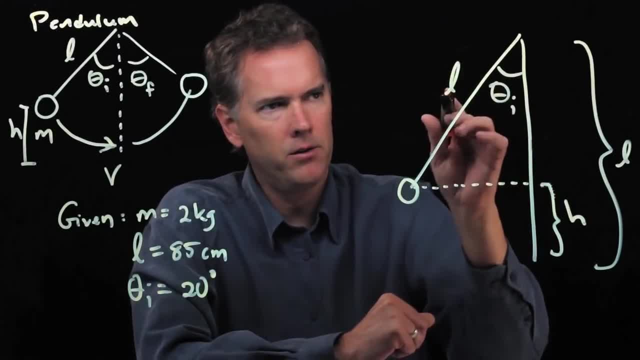 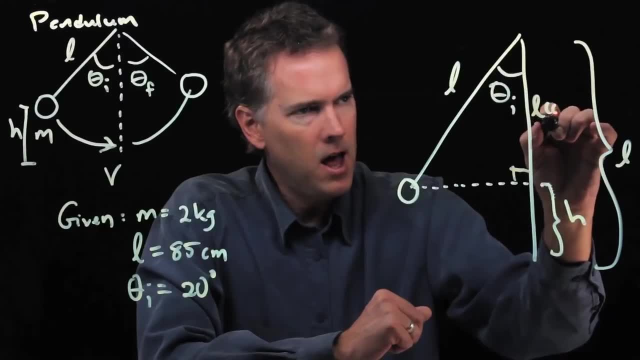 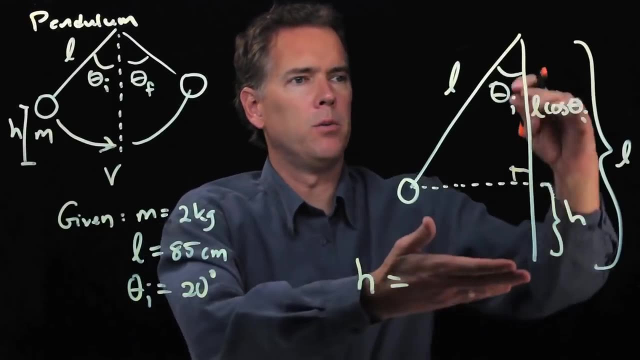 But we know that section because we have the hypotenuse of the triangle. This is a right angle. We have theta i, And so this is l cosine theta i. Okay, so what's h equal to h is equal to the whole length, l. 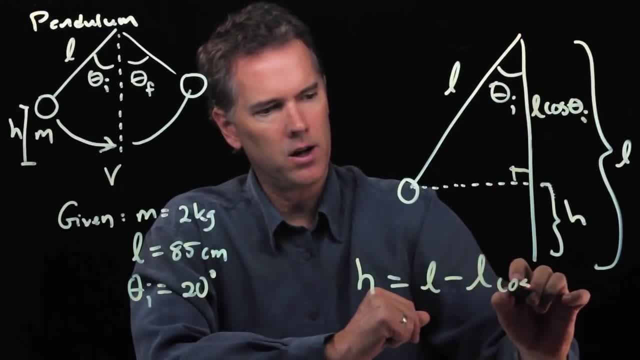 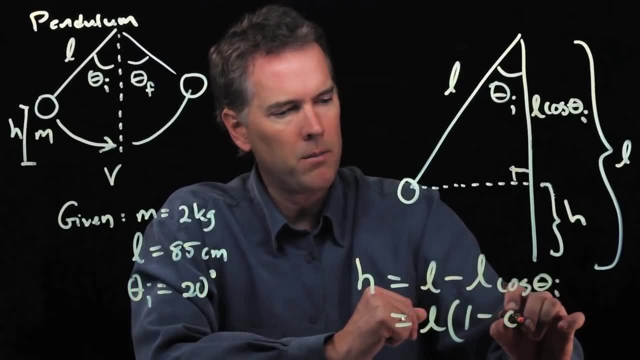 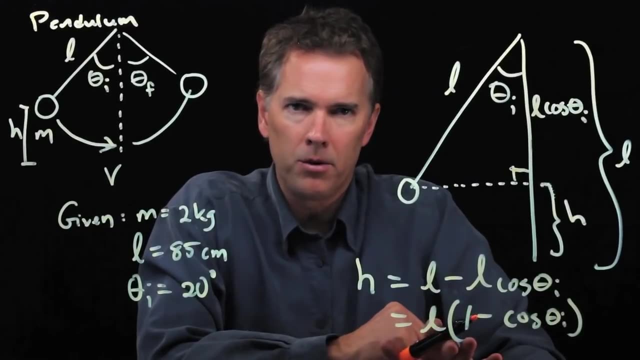 minus this little section, l cosine theta i, And I can simplify that a little bit. It becomes l times 1 minus cosine theta i. okay, And now we have all those numbers and we can plug it in and try it out. 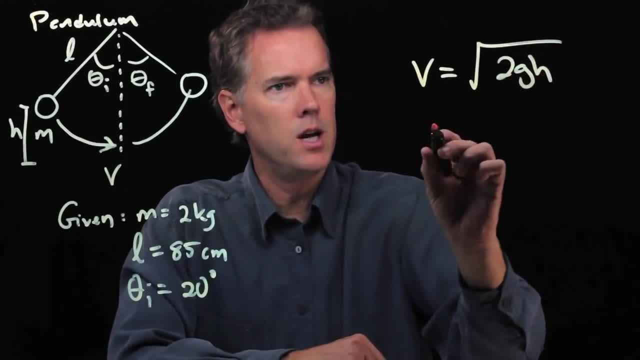 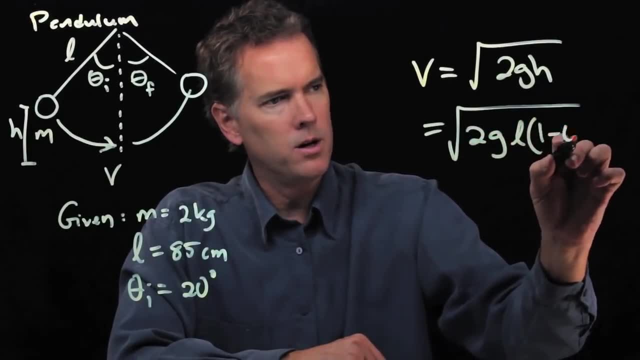 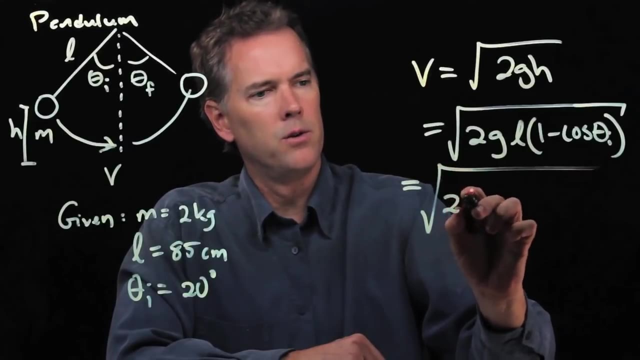 Okay, we said v was square root of 2gh, which is square root of 2g times h, which we just said was l, 1 minus cosine, theta, i, And now we can plug in all those numbers 2 times 9.8 times l, which we said was 85 centimeters. 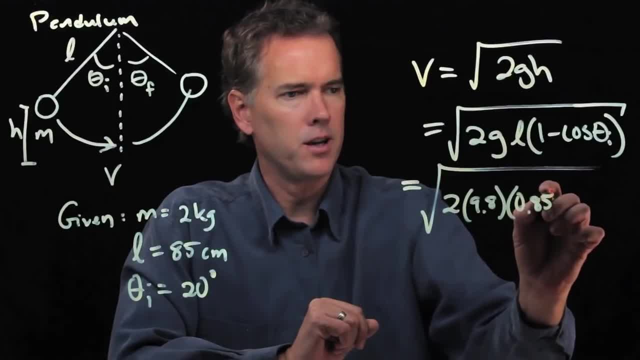 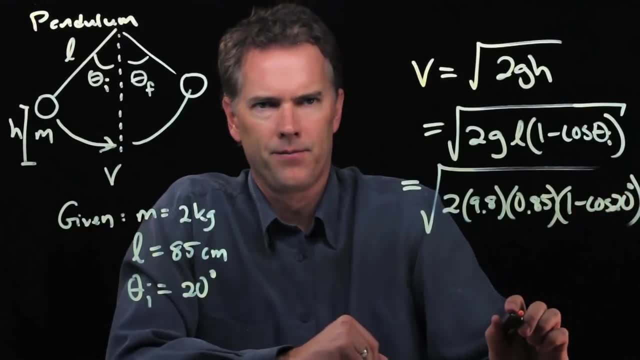 but we got to put in SI units, so that's 0.85.. And then we have a 1 minus cosine of 20 degrees. okay, Plug in all those numbers into your calculator and let's see what we get. 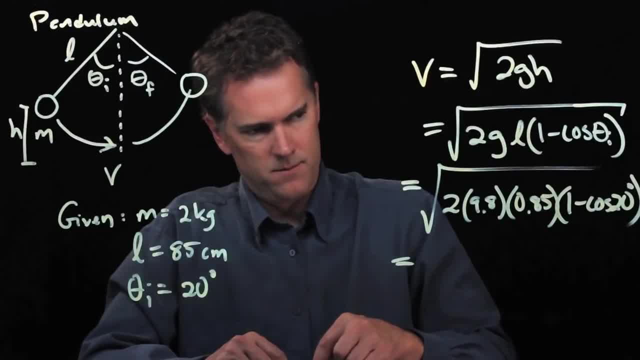 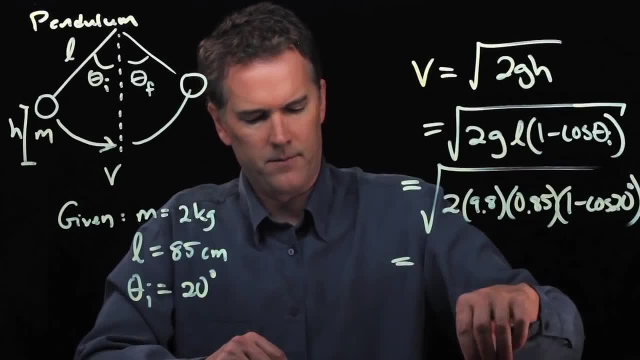 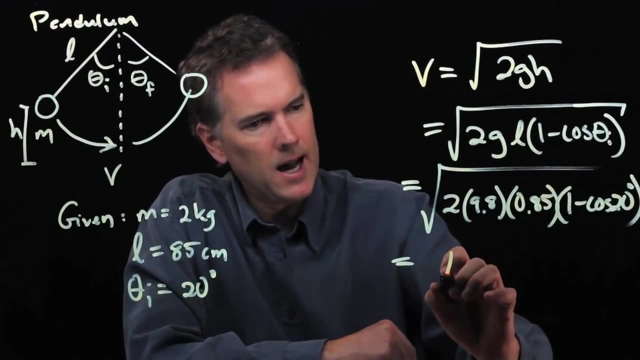 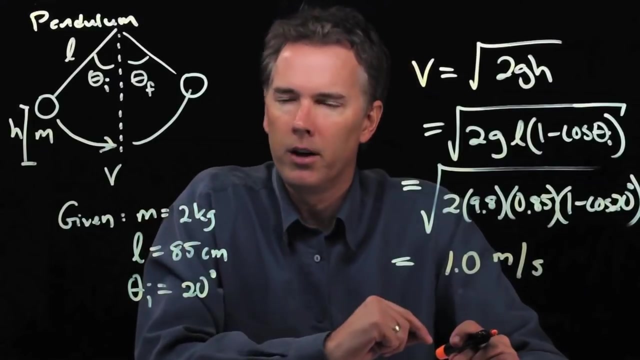 Okay, double check my calculation. but when I plugged it in I got 1.0 meters per second. okay, That's how fast the thing is moving at the bottom of the swing. Okay, by symmetry. earlier we said that theta f. 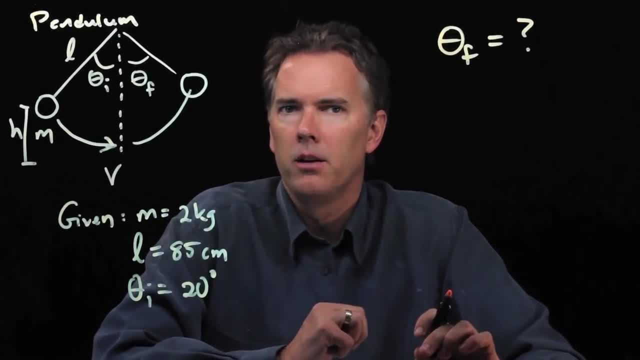 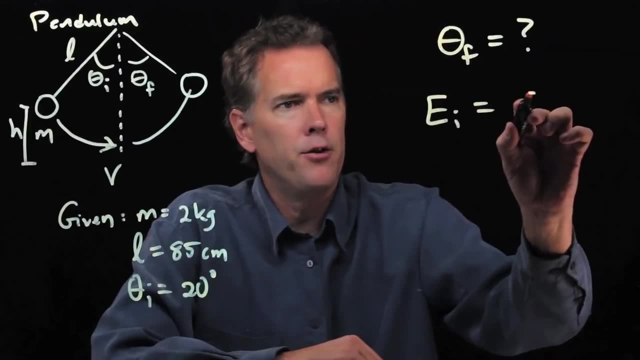 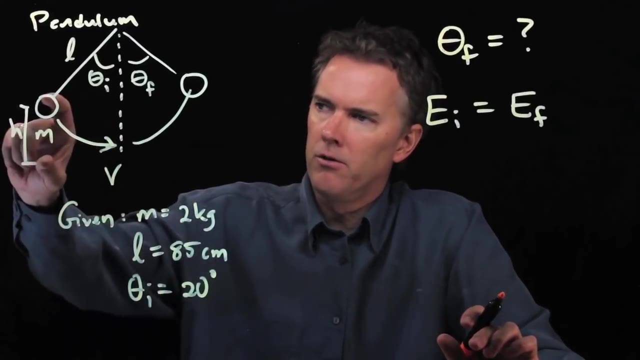 must be equal to theta i. But let's see if we can really convince ourselves of that from conservation of energy. Well, energy conservation says whatever energy we have initially has to be whatever energy is there finally, And if our initial position is there and our final position is there, 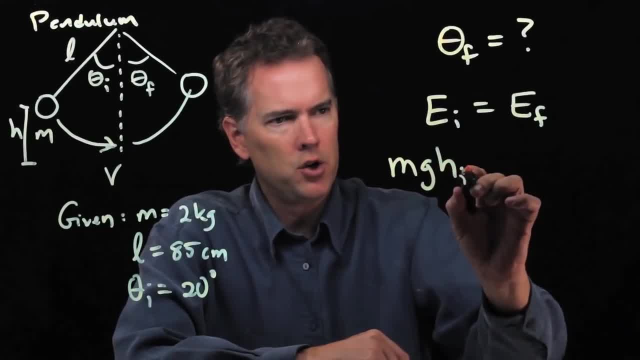 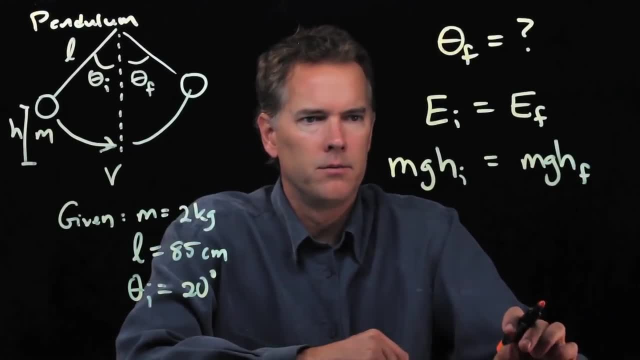 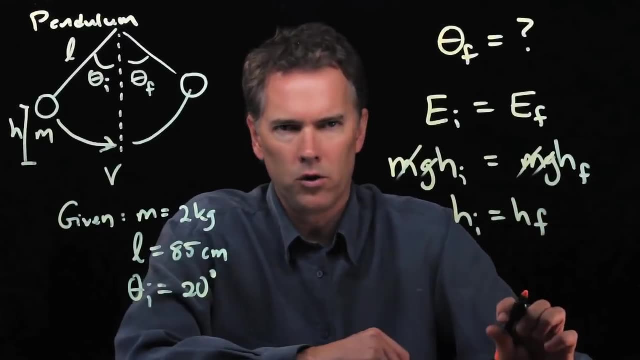 then we just have mgh initial on the left side, is mgh final on the right side, But the m is the same, the g is the same, and so we have to have h initial is equal to h final, and if those heights are equal, we know what that is in terms of the angle.